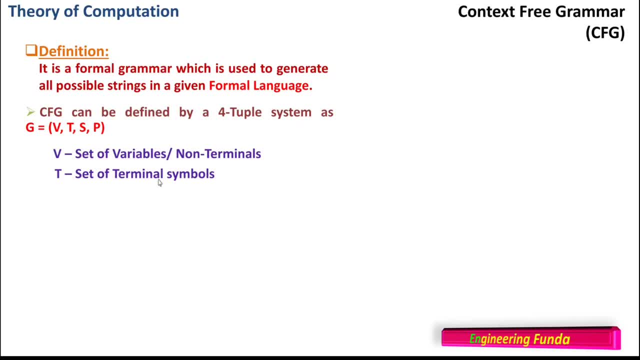 the string T is nothing, but it is the set of terminals. So this set of terminals are the terminals which are formed from the alphabet set. Now, this alphabet set we defined for the language initially, S is the start symbol. So for our grammar we have already seen that we start deriving a string from: 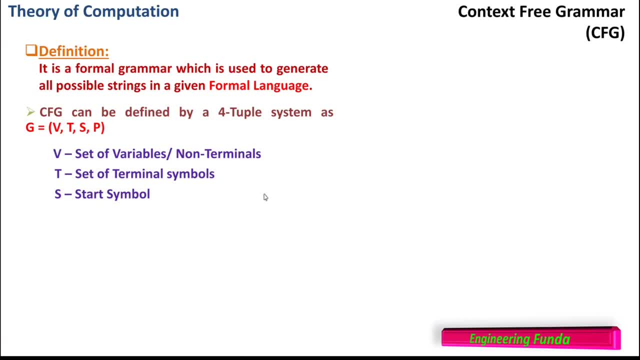 the start symbol, because this is the starting point from where we start our derivation And where P is nothing, but it is the set of production rule where the left-hand side of the string generates the string. Here the left-hand side will not have any right context or left context. 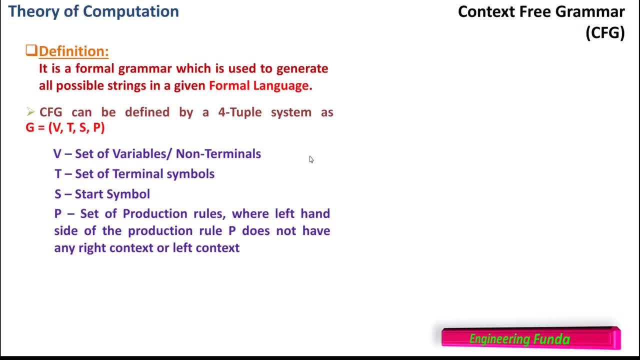 That means, while deriving a string, we don't see the left and right part of the string which is already derived. What we do is we take the non-terminal and use the production that we can use for generating the string. It is of the form A tends to alpha, where a belongs to V. 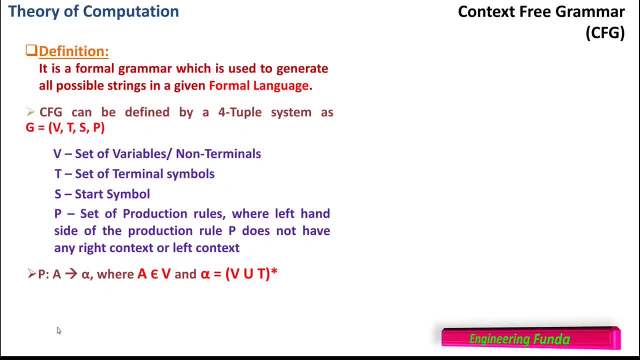 V is nothing but a set of variables or non-terminal. So here we can see that the left hand side is a single non-terminal or a single variable, but alpha is v union t whole star, that is. it is the clean closure of v union t, So alpha. 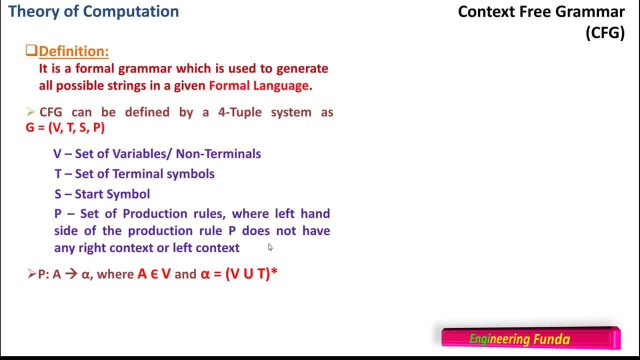 can have any number of variables and any number of terminals. So, as said here, my a is of length one. that means it is a single variable. that is, the non-terminal is free from contact on the left and right side while deriving the string. In CFG the start symbol is used to derive the string. 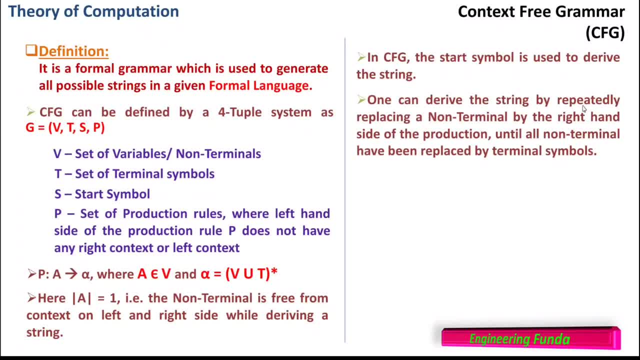 One can derive a string by repeatedly replacing a non-terminal by the right hand side of the production. until a non-terminal is used, all non-terminal have been replaced by the terminal symbol. this derivation we have already seen in the previous video, my dear friends, where we try to derive a string from the given grammar. 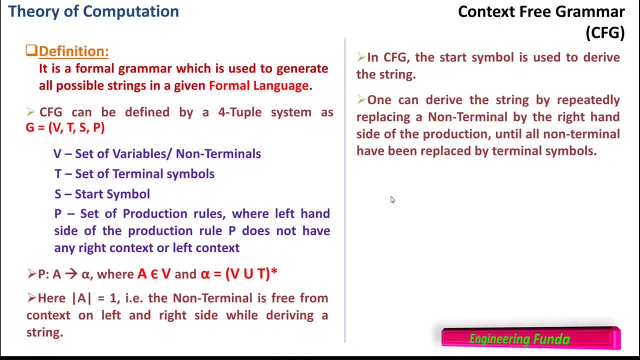 in which what we used to do is: we take a production, we select a non-terminal from the production and try to explore it by replacing it with the right side of the production, which contains the non-terminal on the left hand side, and we continue this process for deriving a string. 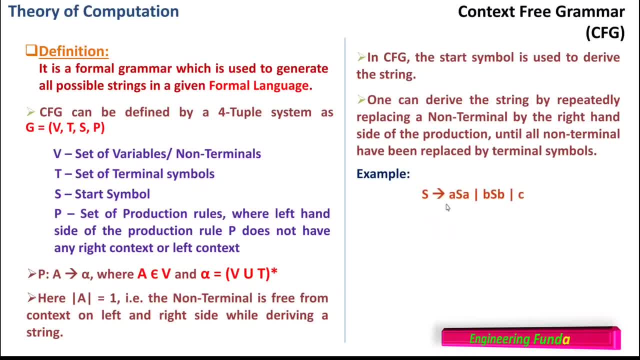 let us repeat this with an example. let us say that there is this grammar given to us, where there are three productions: s tends to asa or s tends to bsb or s tends to c. here this s is my starting symbol: s tends to asa is one of the production, s tends to dsb is another production, and s tends to small c. 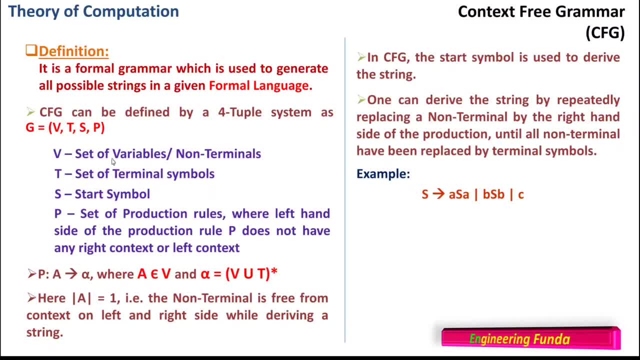 is my third production. my set of variable or non-terminal contains only one letter, that is s, and my terminals here are a, b and c. let us try generating the string a, b, c, b, a using this grammar. my dear friends, we can observe this from this grammar, that the non-terminal is in the between. 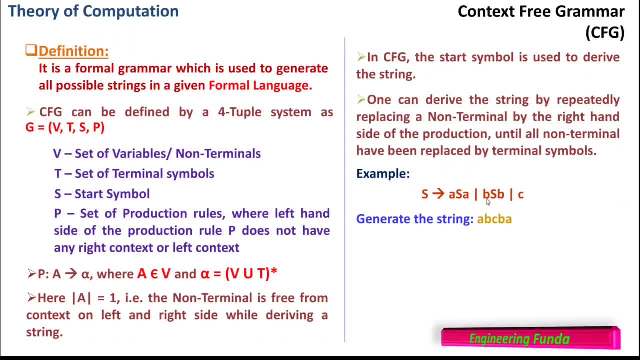 in this production it is between 2a and in this production it is between 2b. so while generating this string, we can see that the first and last letter are a. okay, so we have to use the production s tends to as a, because whatever will be added will be added in the place of this non-terminal. 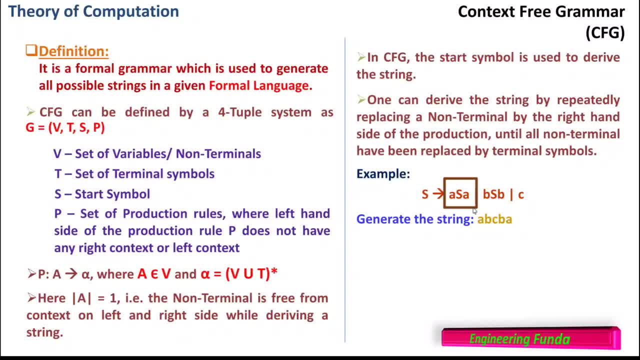 s. so my first and last letter, the first production that i use, will give me my first and last letter. so if i use this bsb, then my first and last letter will be b, but what i want is first and last letter should be a. hence what i am doing is i am using this production s. 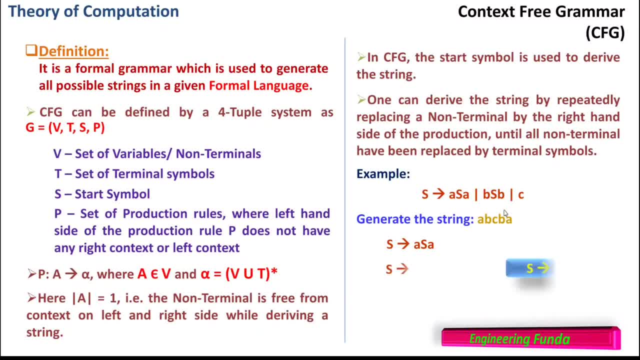 tends to asa. now i know that the second letter and the second last letter i need is b, so i replace this s by this production s tends to bsb. my first and last a will remain same and this s will be replaced with bsb, so hence it is giving me this pattern. and now in the 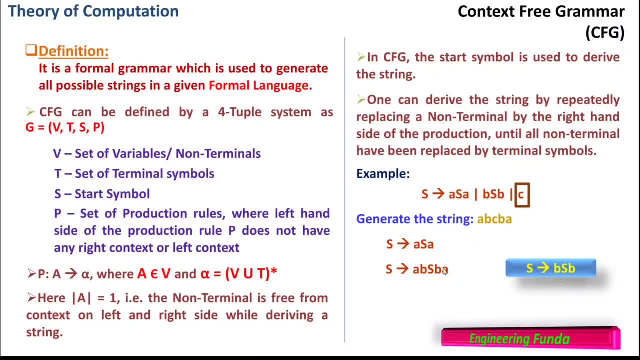 next step. i want this c to be there, so i will use this production- s tends to c- and i will be able to generate the string abcba. i hope it is clear, my dear friends, because it is the use of this production, the order of the use of this production, that defines what string you. 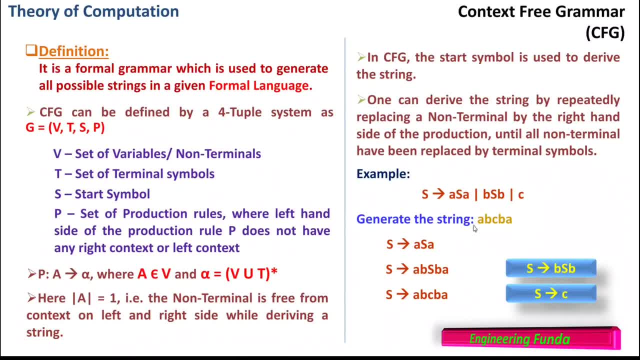 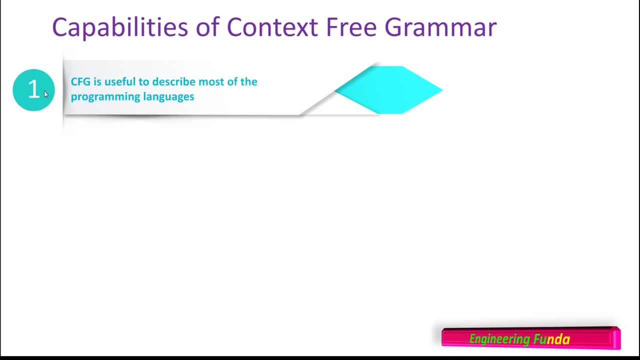 are going to get and, depending on the string that you are going to generate, you have to use this. production rules one after another. now let us see the capabilities of context free grammar. the first capability says that cfg is useful to describe most of the programming language. by using cfg, we are able to describe most of the programming. 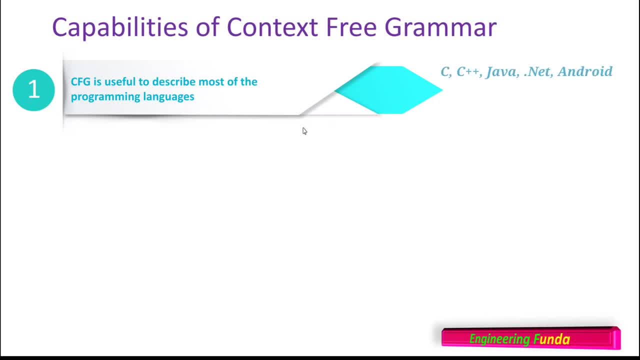 language: c++, java, dotnet, android, any programming language. there is a context free grammar written for that language using which we check the generation of any string. to give you a simple understanding, if we are checking whether my expression is correct or not in c language or c plus plus, 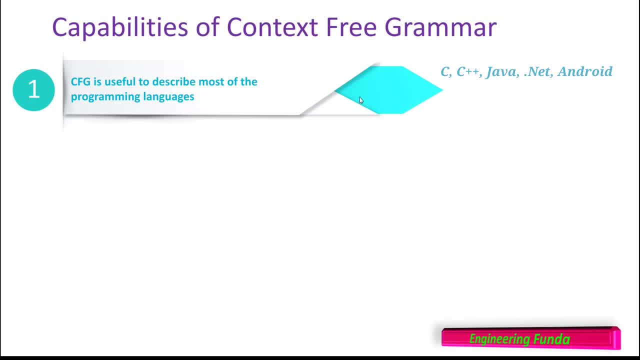 then we know that my expression ends with a semicolon. so i can write a semicolon and in its form i can write a grammar for that. of the form, a tends to alpha where there is a semicolon at the end. the second capability says using the features of associatively and: